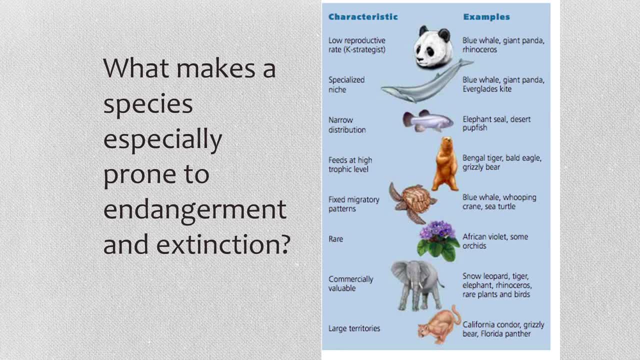 cause you to have less Ability to compete. Narrow distribution if it feeds at a higher level, on the trophic level, if it has fixed migratory patterns, if it's rare, if it has commercial value to it or if it is. 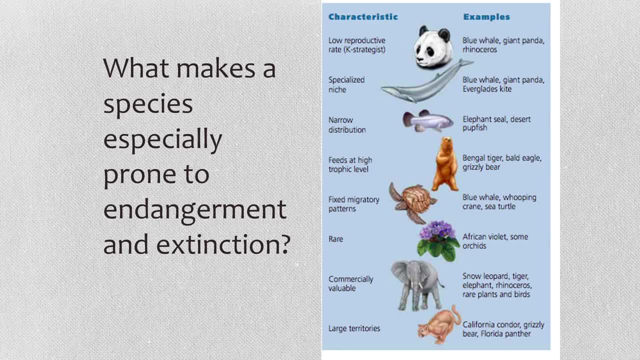 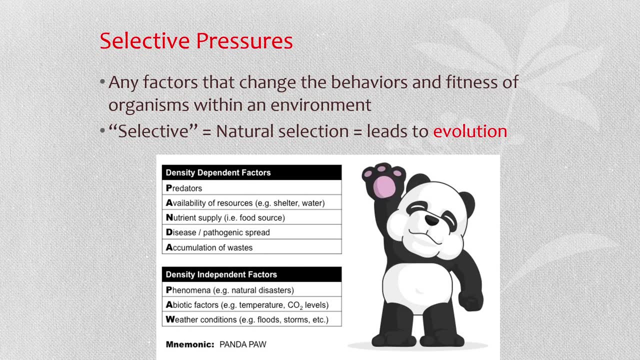 a species that takes up a large territory. These are all things that could cause endangerment and extinction or make them more prone. So selective pressures are just factors that change the behavior and the fitness of organisms within an environment. Selective, like natural selection, is a factor that changes the behavior. 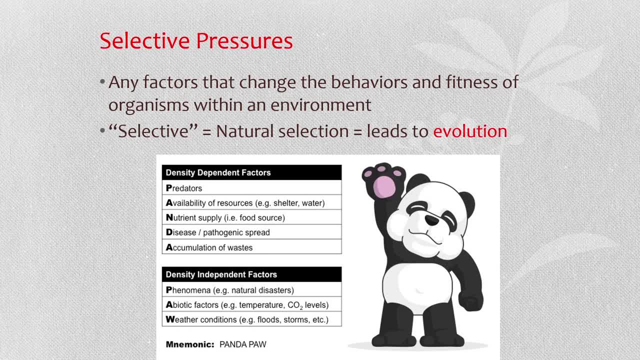 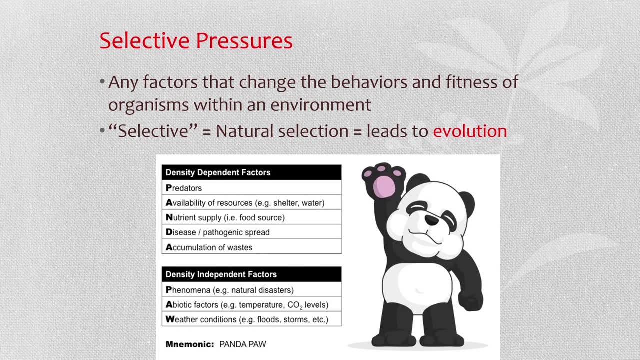 and the fitness of an organism within an environment. Selective, like natural, selection, will lead to evolution. Density-dependent factors versus density-independent factors. The density-dependent factors are panda predators, availability of resources, nutrient supply, disease or pathogenic spread and then accumulation of wastes. Density-independent factors are: 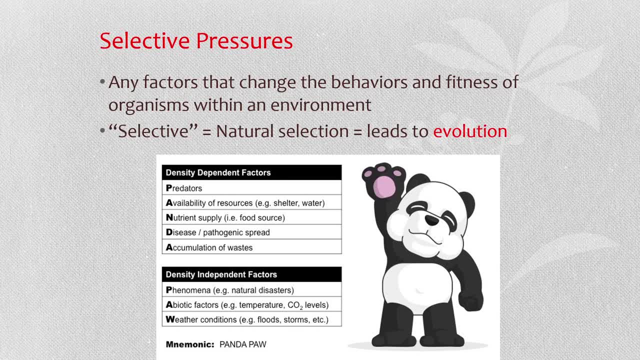 phenomena like natural disasters, abiotic factors such as temperature, CO2 levels and then weather conditions. So if it has a low reproductive rate, it's going to cause it to go endangered If it has a Dependent density- dependent just means if there are more of them, these are going to cause more. 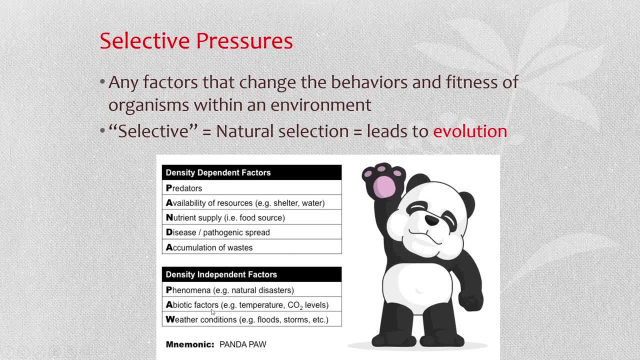 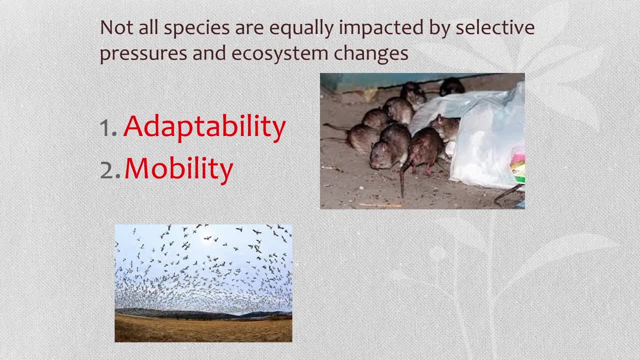 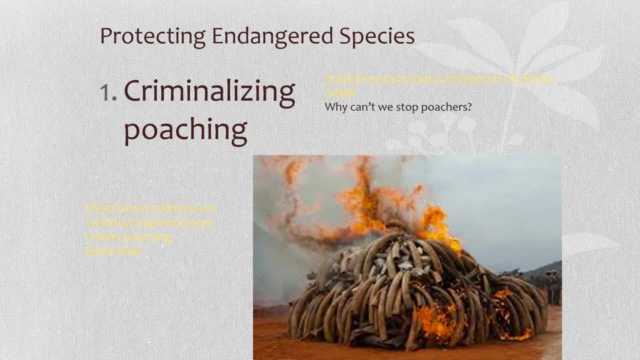 problems, Whereas density independent. it doesn't matter how many of the species there are, these will affect them. Not all species are equally impacted. Some species have better adaptability and mobility, which allows them to thrive or do okay. So the protecting endangered species. 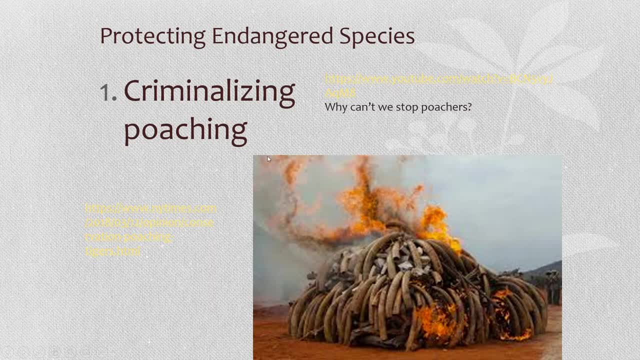 there's different ways that we can do it, like criminalizing, poaching. So it's a super sad picture. There's a video here you can and a video here, an article here and a video here. you can actually check those out if you click on the link inside of the PowerPoint which you can. 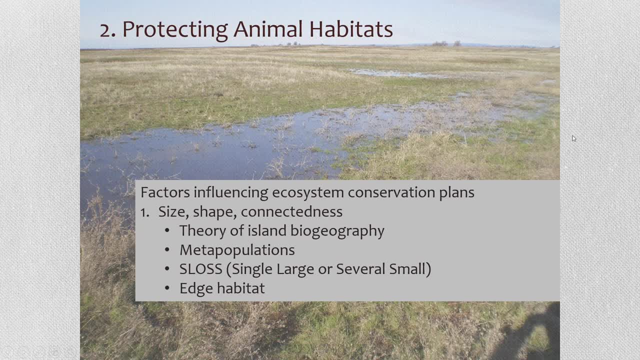 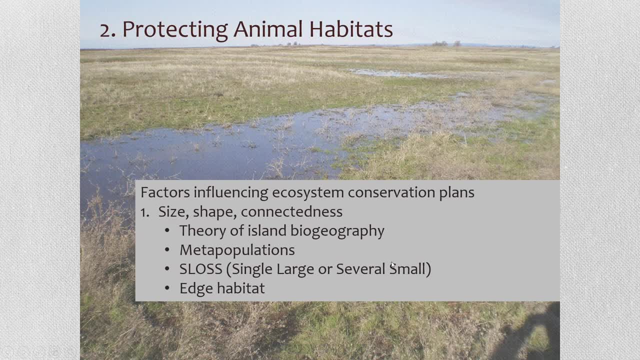 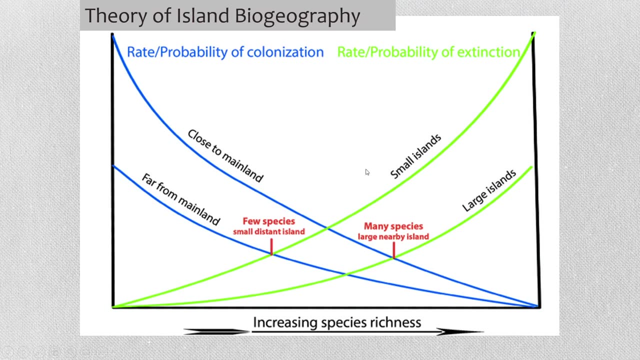 Consideration metapopulations- single, large or several small and edge habitats, And we'll talk about that all in a second. So here you go. Remember island biogeography, where their ability to migrate based on large island, small island if they're close to the mainland or far from the 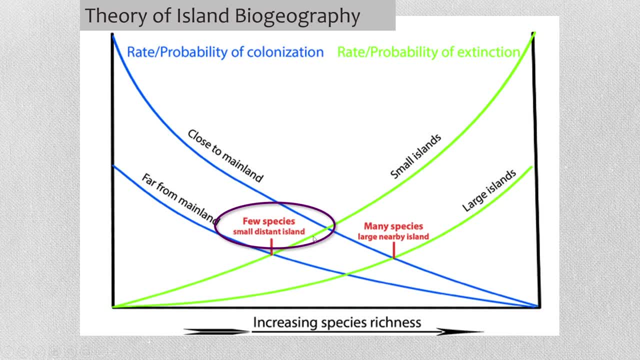 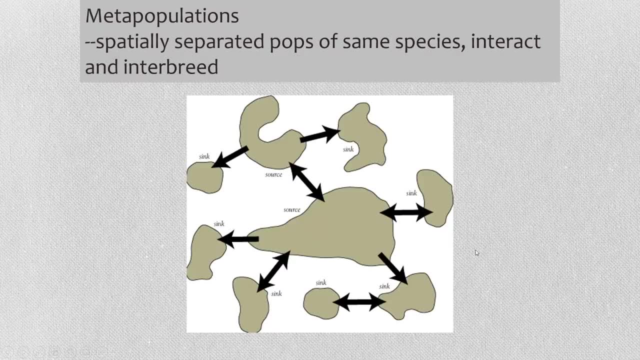 mainland. If they have a few species that are going to be on a small distant island, there will be many species on a near a large nearby island. Metapopulations is where you have spatially separated populations of the same species which interact and interbreed. Sorry, Oops, Yeah. So the ability to go across, like these different 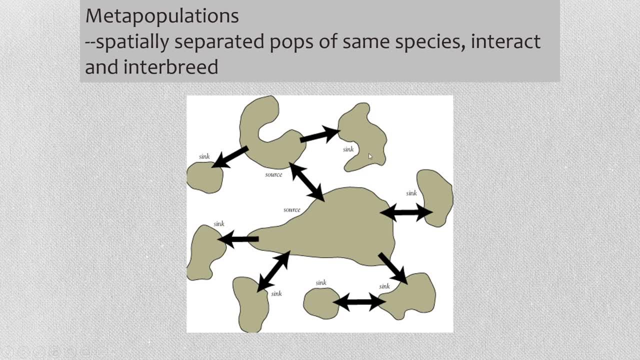 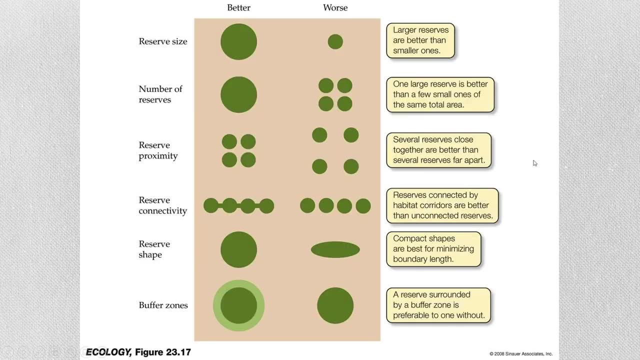 islands, they're able to interbreed and interact with the same species. If they're farther away, obviously that's going to become less of a problem or it's going to become less likely. We can also see that if we create large reservoirs versus small reservoirs. large reservoir is always. 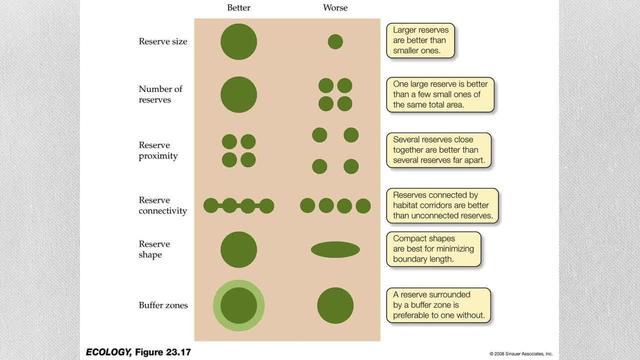 bigger than a smaller one. One large reservoir is going to be better than a few small ones in the same total area. If you do end up going with small reservoirs, you don't want to space them too far. You want to try and keep them as connected as possible, giving them habitat corridors. 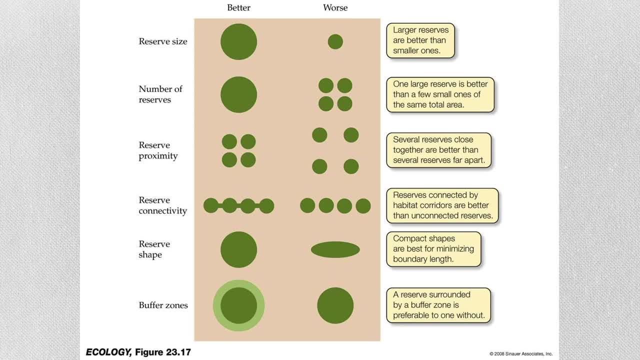 because then you can have their ability to go from one to another. Typically, if you have a complex area, you're going to want to keep them as connected as possible, giving them habitat corridors, because then you can have their ability to go from one to another. Typically, if you have a 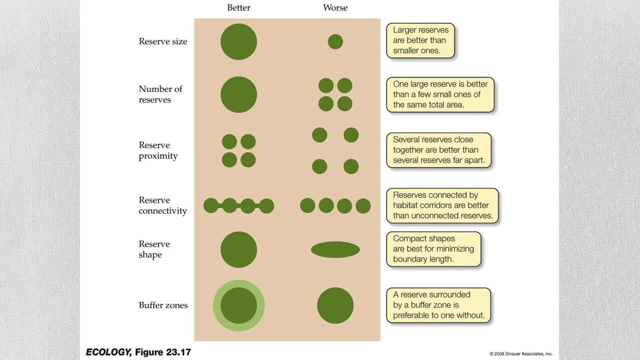 compact shape. it minimizes the boundary length, So this right here has a less of a boundary length than this right here You also want to create buffer zones, which is an area that allows for a slight amount of buffer with the environment outside of it. So when you're creating these, 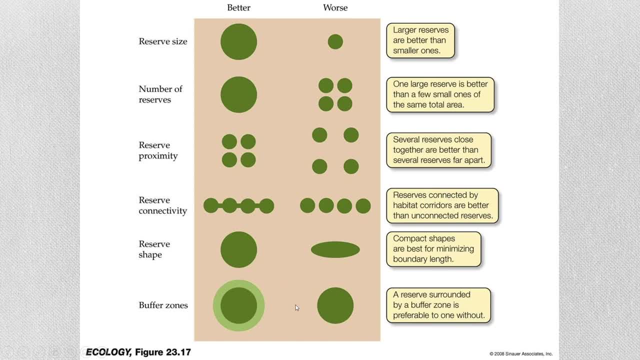 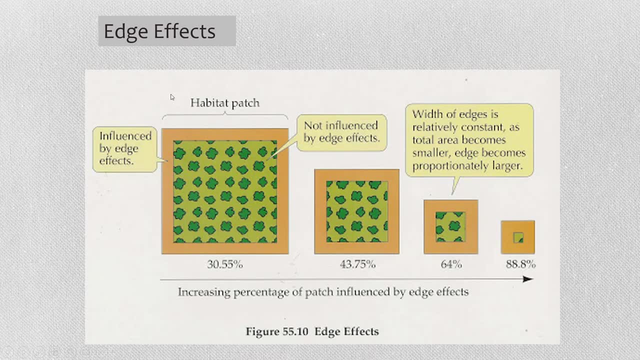 reserves. if you ever get into the business of creating reserves or if you want to create a solution where you say we need more reserves, these are things that you can keep in mind. Edge effects are important when these reserves are put into place. So, for instance, if we have 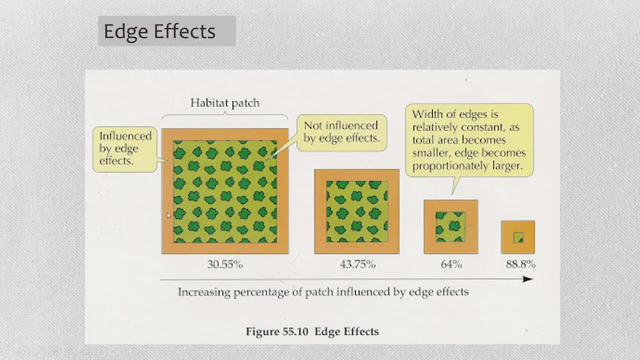 plants out here, these are going to be affected by edge effects- the species that are on the outside of this preserve. So if you have an increasing percentage of the patch being, you'll have an increase percentage of the patch being affected by more of edge effects. So inside they're not. 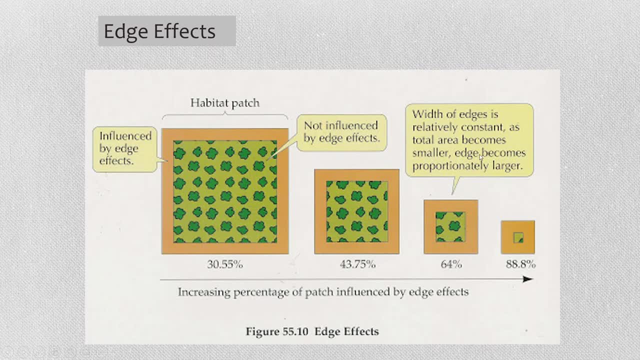 going to be affected. On the edge they are affected. On the inside they're not going to be affected. The width of the edges is relatively constant, So if you have a larger area you're going to have less of an edge effect. So creating a bunch of small zones like this you're not going. 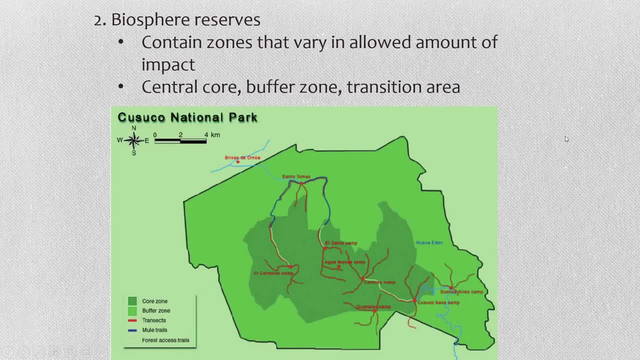 to get as much as creating one large zone. You also have to consider biosphere reserves. These contain zones that vary in allowed amount of impact. You can have a central core, the buffer zone and the transition area. So whenever there are reserves, these are things that have to be. 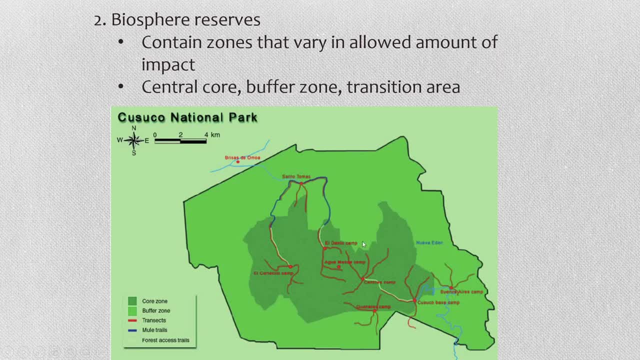 taken into consideration. Looking at water, traveling through the core zone is in the middle. The buffer zone is on the outside. The transects are inside of the area where you can transfer from one area to another. This is just one example of Cusco National Park. So whenever they create national parks or national 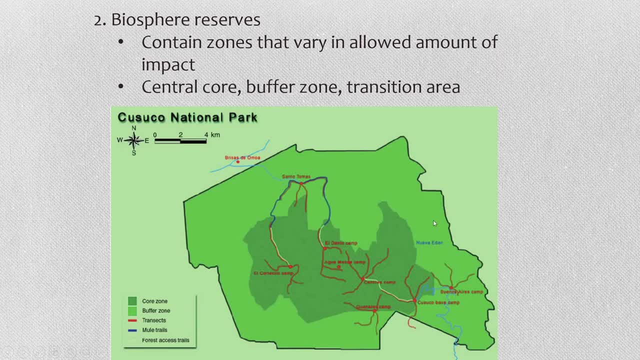 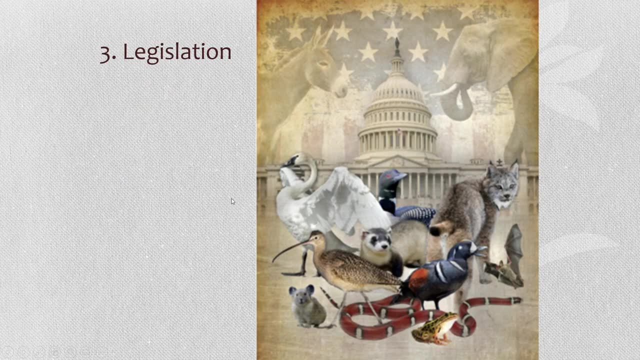 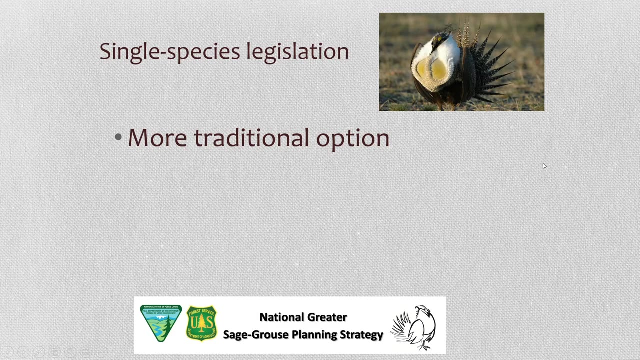 wildlife reserves. these are all things that they make sure to consider. That's why they're much larger usually than what you would expect them to need to be. We can also do things like legislation to help prevent endangered species, So there are examples of single species legislation. This is like the more traditional 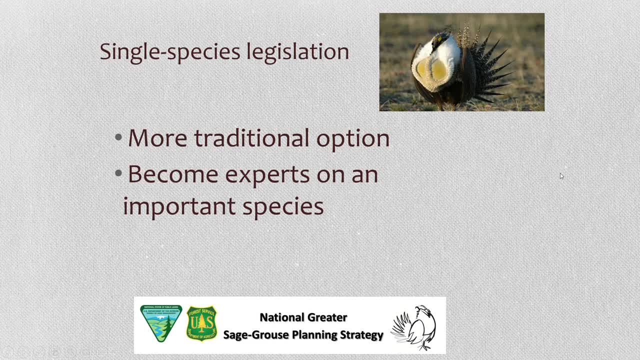 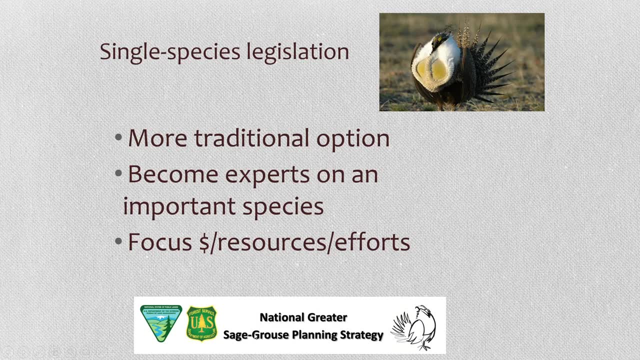 option because people become experts on an important species and they can focus their money and their resources and their efforts. So, for instance, the national greater sage-grouse planning strategy to protect the sage-grouse right- One species much easier to focus on. one. 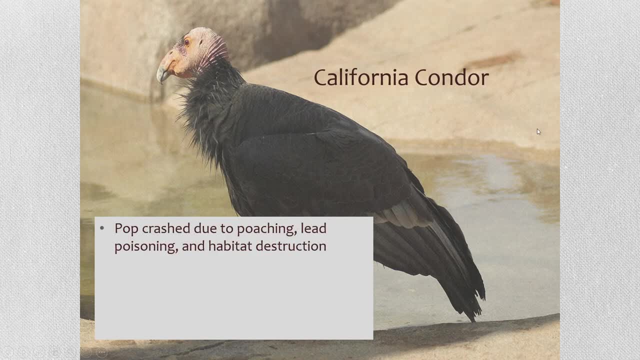 species. Another example of this is the California condor. Their population crashed because of poaching and lead poisoning, as well as habitat disruption. They could not use thegendjaize because of the safety of this species, but they are learning new techniques and doing nothing, And I would look. forward to seeing their longtime history. This is a great question for further discussion next year, so I'll just stick to it. I know the next question and I hope you all get excited about these topics- in the comments and after the break. Okay, And probably be able to give some comments about it. 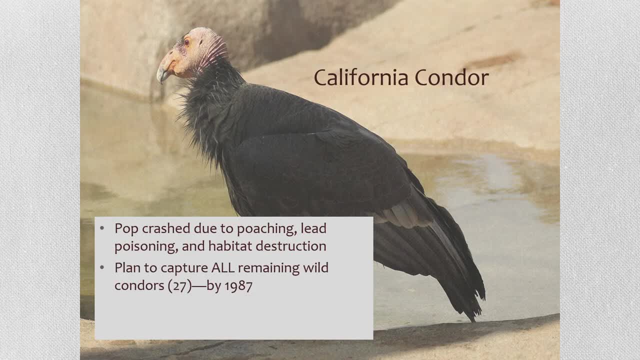 destruction. there was a plan to capture all of the remaining wild condors. there were only 27 by 1987, and then they had captive breeding and reintroduction. they are now 400 to 500 in the wild today. so another example of a single species where we can try to protect one species. so the 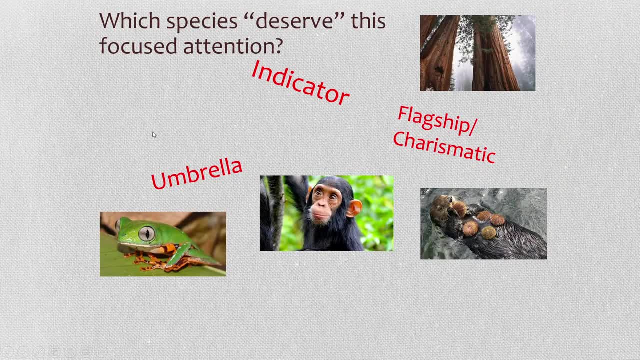 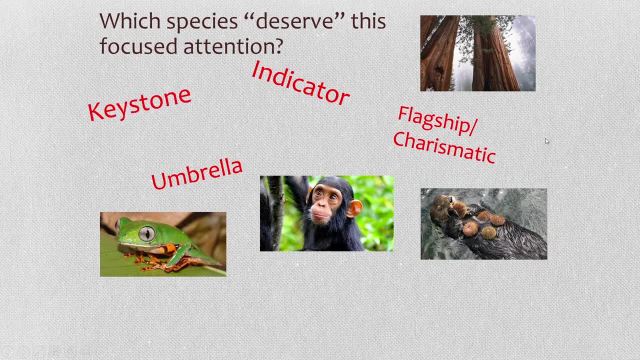 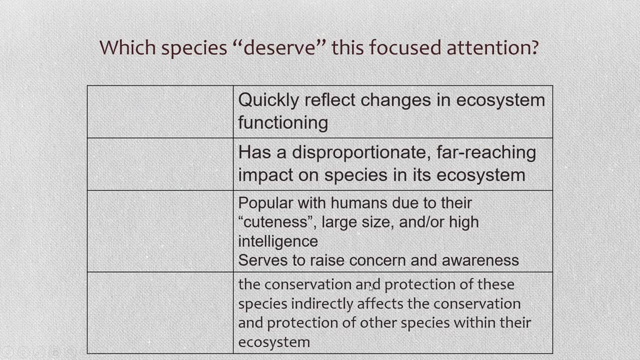 question then becomes: which species deserves the focused attention? do we protect the umbrella species? do we protect the indicator? do we do we protect the flagship or charismatic species, or should we protect the keystone species? so just a reminder of some of those definitions of these types of species quickly reflect changes in ecosystem functioning. hopefully you know that's. 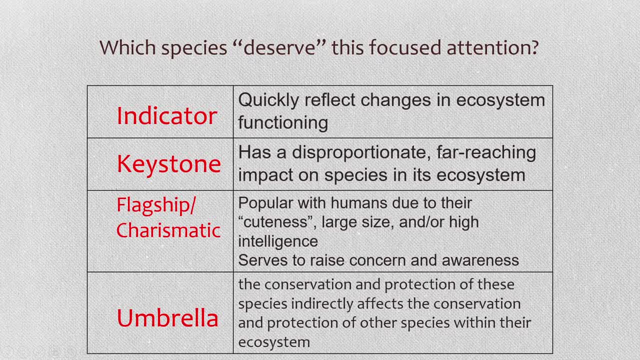 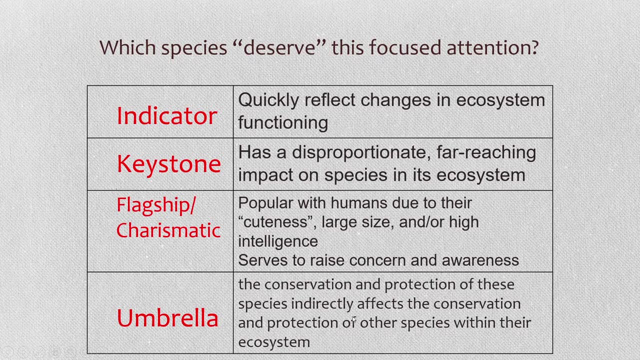 an indicator species keystone has a disproportionate, far-reaching impact because it is the keystone. a flagship is popular with humans typically based on cuteness, large size or high intelligence, and that can raise concern or awareness. and then umbrella is the conservation protection of these species indirectly affecting the conservation and protection of other species within their 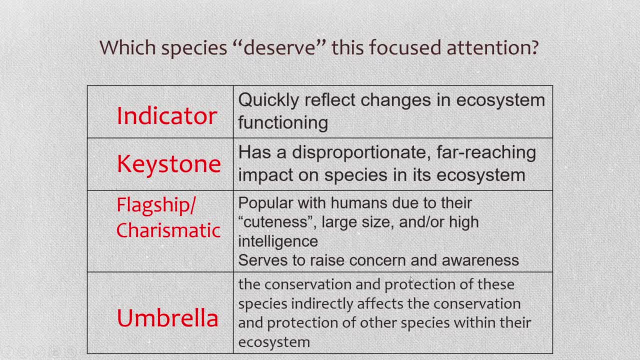 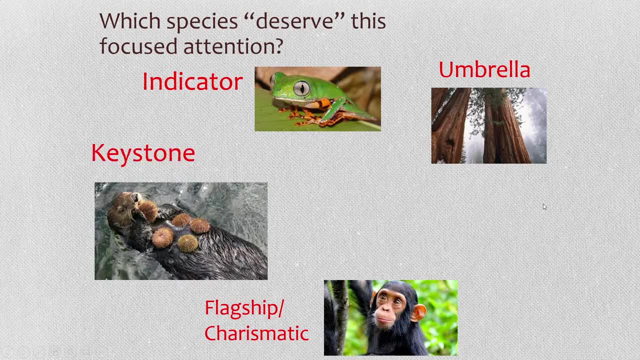 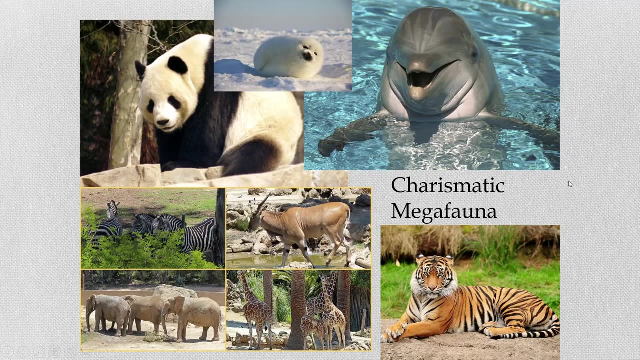 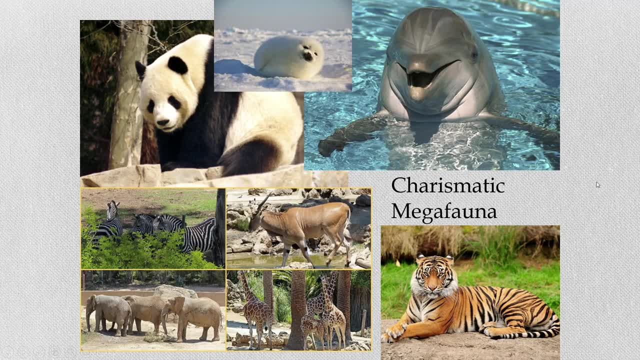 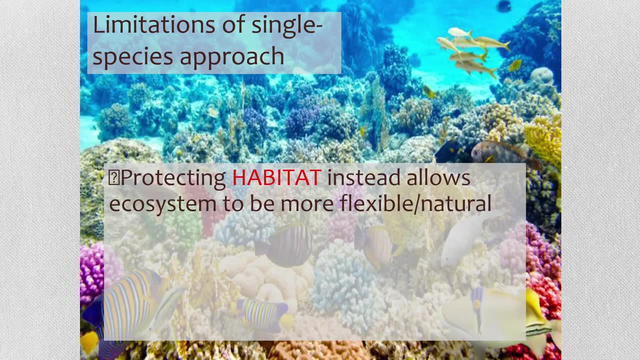 they're pretty, we like to see them, we like to. you know, we want to pet them, so we try to protect them. some of the limitations of a single species approach, of course, is that if we don't protect the habitat, we're not really doing much. if we can protect the habitat, we're allowing more flexible. 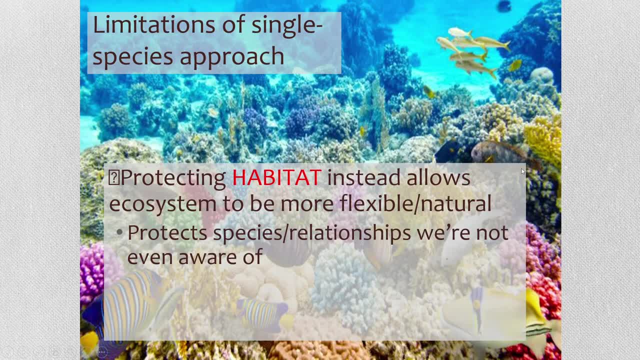 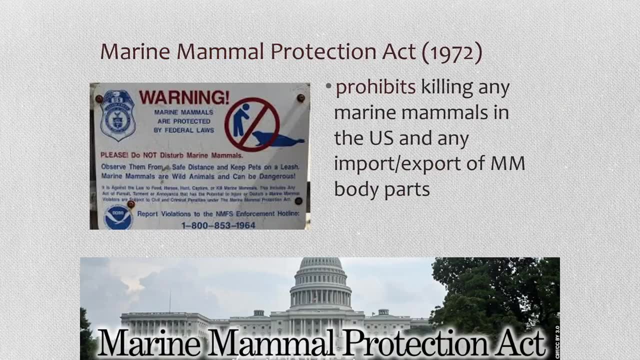 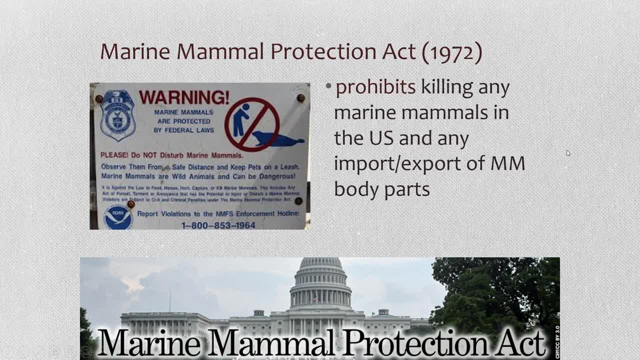 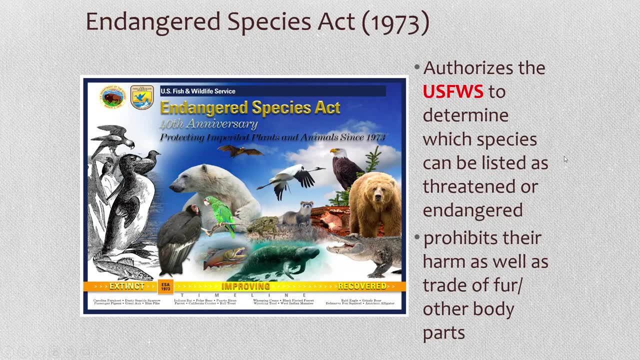 Mammal Protection Act, which prohibits the killing of any marine mammals in the US and any import or export of marine mammal body parts. The Endangered Species Act was put into place in 1973, which allows the US Fish and Wildlife Service to determine which species can be listed. 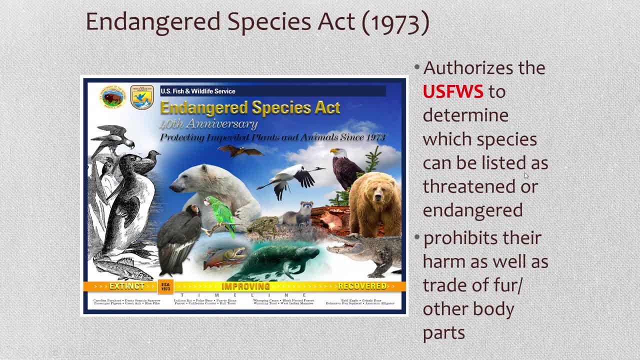 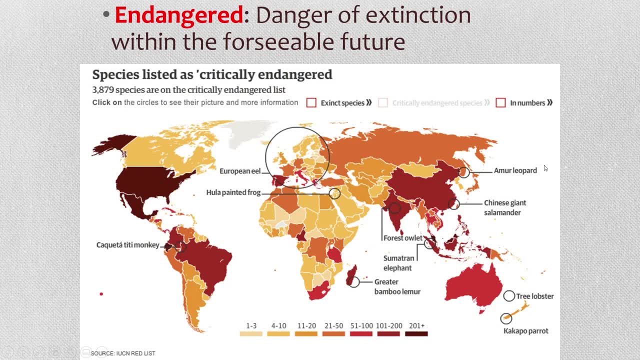 as threatened or endangered and prohibits their harm, as well as trade of fur and other body parts. So what is endangered? Well, endangered just means that it has a danger of extinction within the foreseeable future. So this is an example of a map of species that have been listed as: